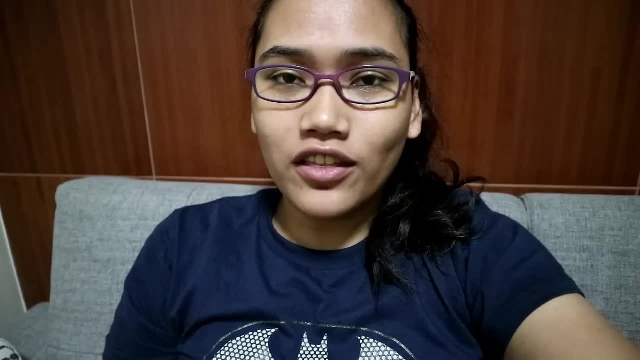 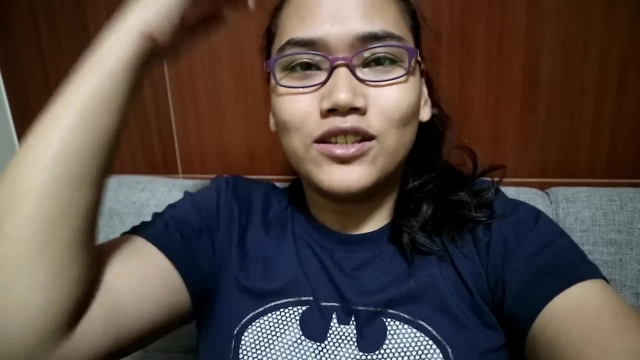 Hi everyone, Thank you for checking out my channel. Thank you for clicking on this video. This video is part of the series of videos I'm posting to try to help people out when it comes to aptitude tests like the civil service exam. It's: 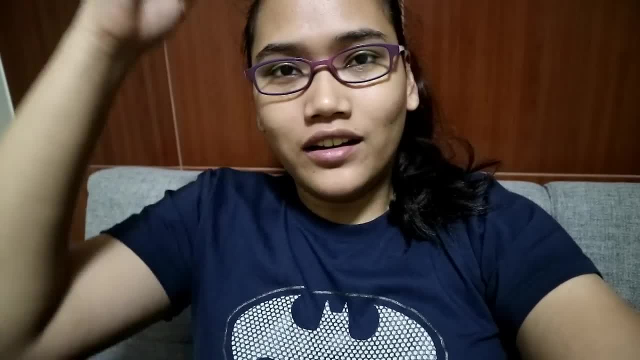 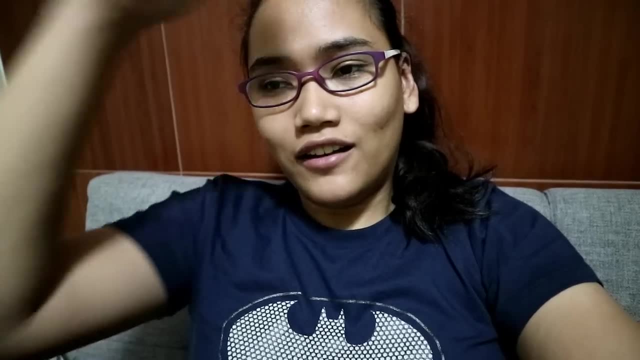 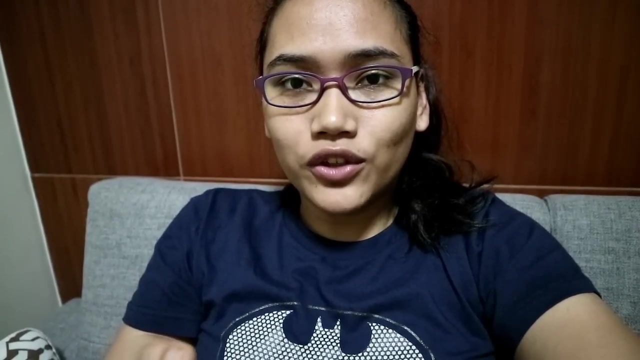 quite late at night right now and I am actually sharing an Airbnb with my sisters because we're hanging out, because I'm leaving tomorrow for a conference and I've been really busy the past few weeks. Sorry about my voice- Again, it hasn't returned in full, but I really wanted to make this video for you because I 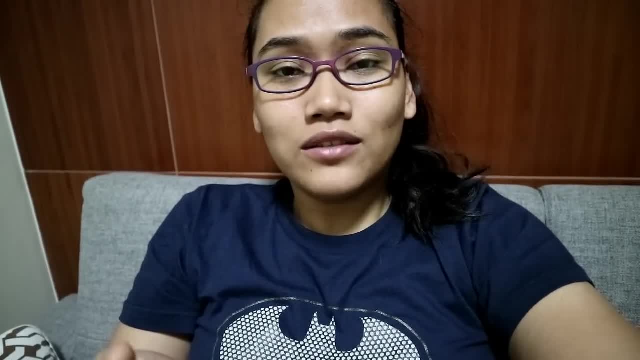 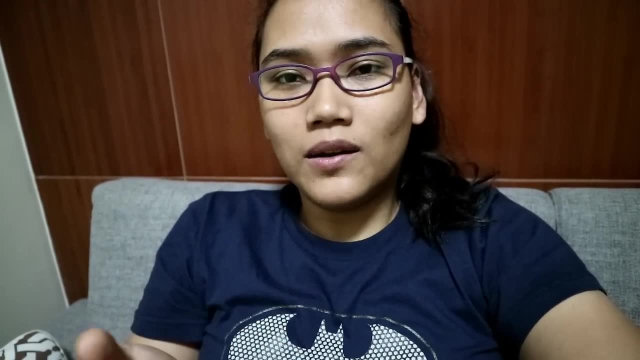 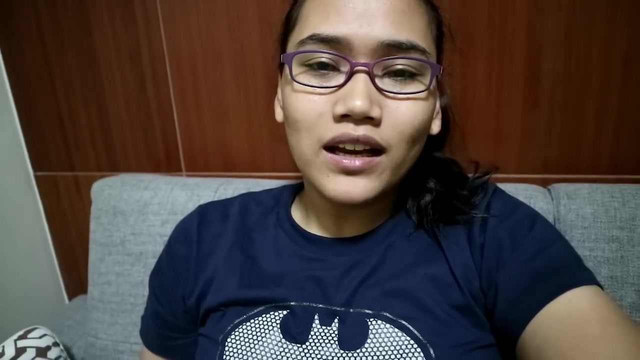 promised you guys that I'm going to make it. This is a by-request video with questions that you sent in through the Facebook page and through the post that I made asking you guys to send in your questions so I can make a video about these. This tradition of Team Laika has been going on since. 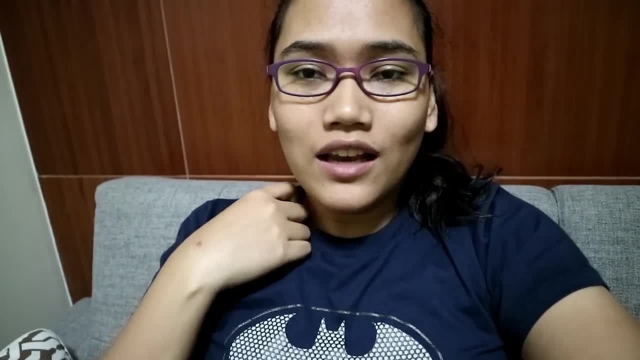 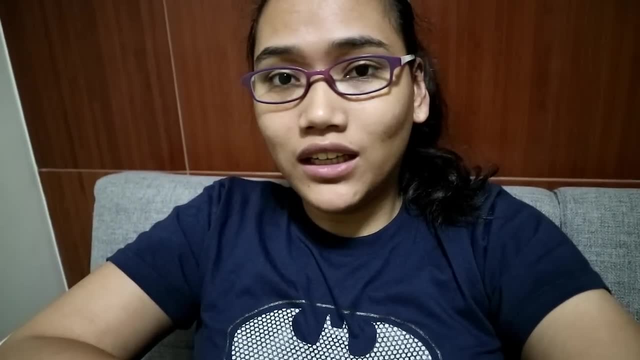 the beginning, When I started making videos, I'd never really planned I'd have my own YouTube channel, Facebook page or anything like that, or even for the reviewers. I'd never really thought that I was going to do that. The only reason why that started was because my students 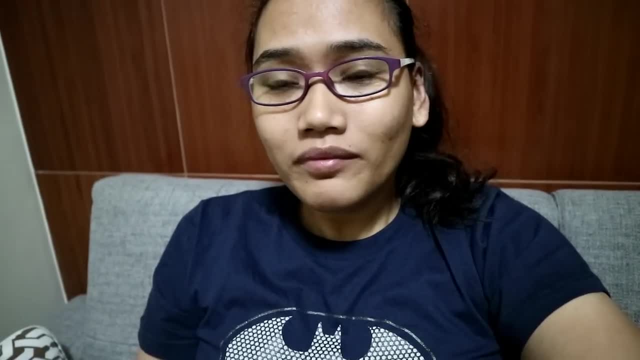 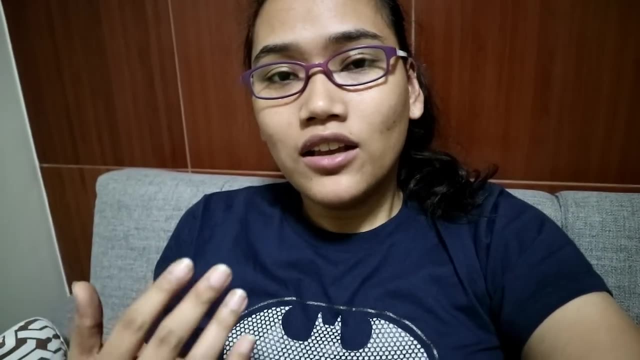 kept requesting that coach, do this, do that. Now this request videos. it started with that because what happened before, when I was just starting out, is that the people that I help from all over the Philippines. they send questions in like coach, how to? 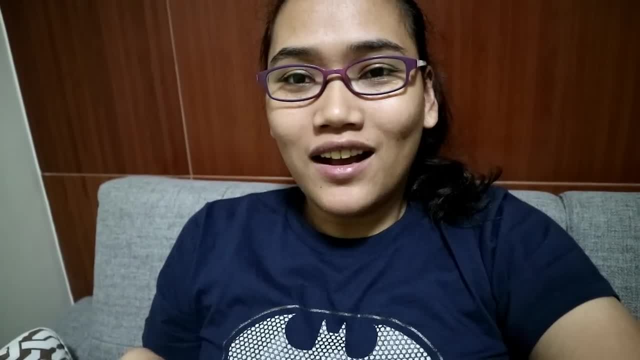 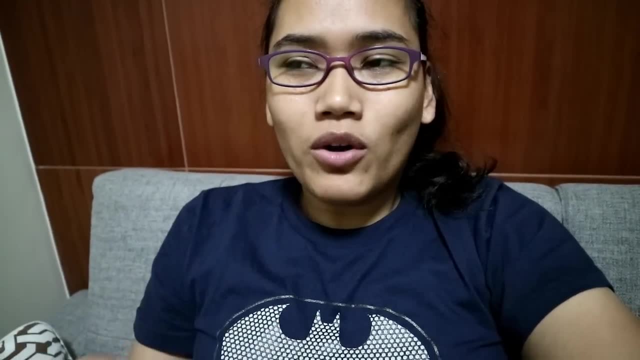 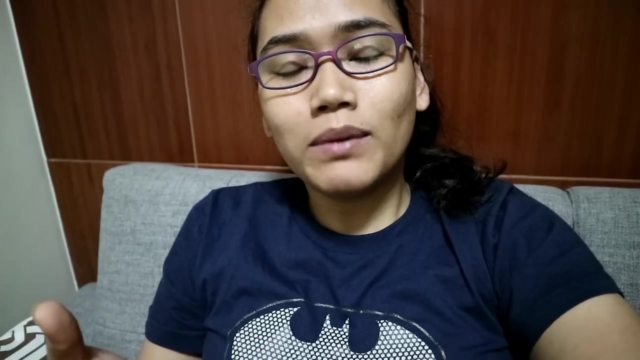 solve this, Or they don't call it coach yet, ma'am, panon or miss, They send me questions, I'll answer myself and I'll post it on YouTube. So I wanted to like revive that tradition so that our learning will be more interactive. So again, thank you to those who sent questions. 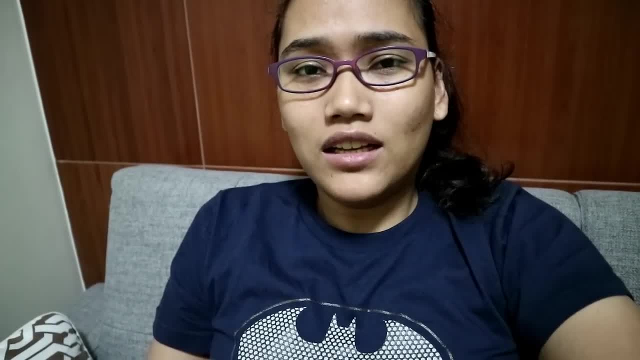 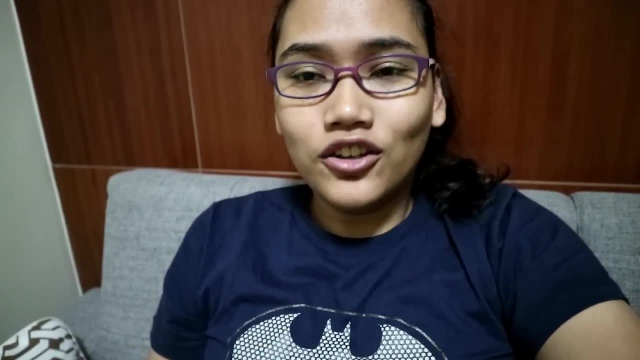 I'm going to try my best to solve all of those that you sent in the limited time that I have. I'm just squeezing this in because my sister is sleeping And there, So while they're sleeping, I'm making videos. So thank you, guys, and I'll see you in a bit I'll show. 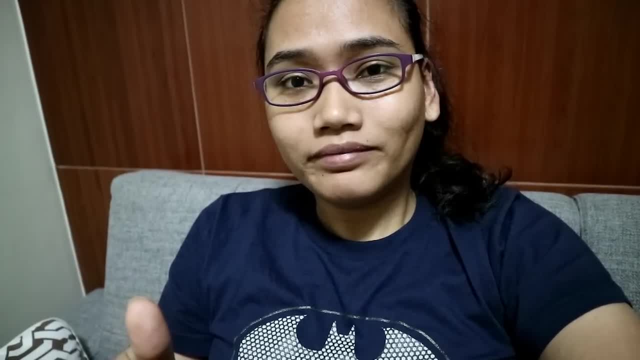 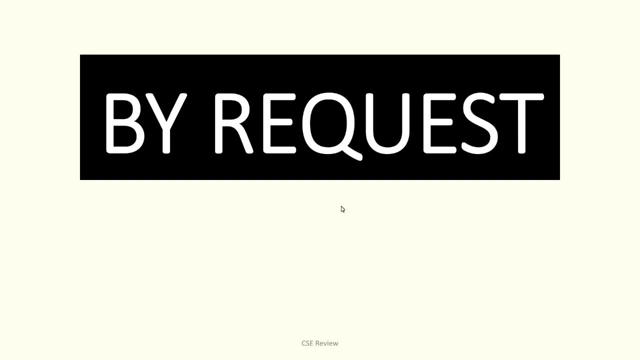 you what questions I have. As I promised you guys, I'm going to make a by request video. In this video, ang sasagutan ko are the questions that you guys sent in. I asked if kung meron kayong mga specific. 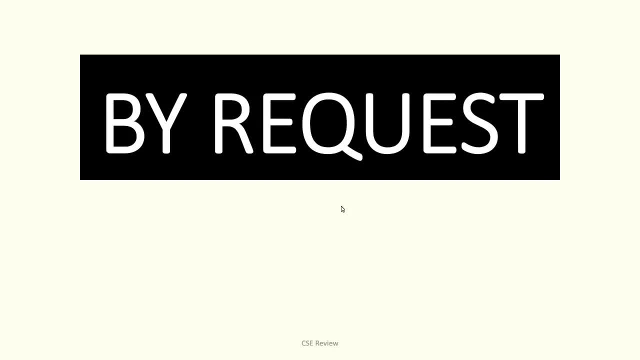 questions that you encountered na hindi nyo alam ko paano isolve ko, paano nyo sisimulan, isend nyo sa akin doon sa post that I made. So that is what we're going to answer ngayon. 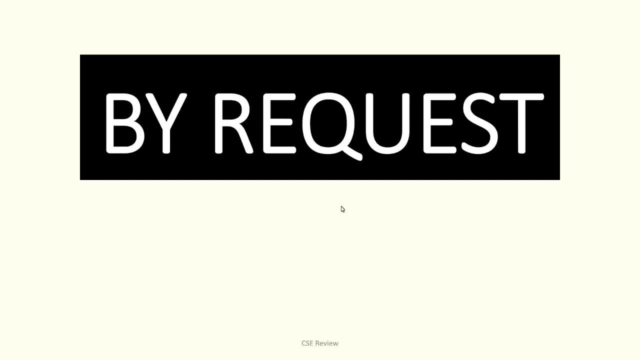 Now these are compiled from those Comments and some of the other questions na pinadala sa akin. na tingin ko makakatulong sa inyong lahat. Okay, Now, I do encourage that you send questions sa akin. You can post. 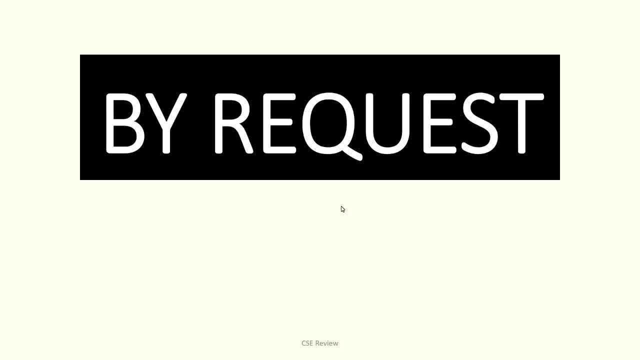 them as a comment dito sa baba or doon sa actual post ko sa Facebook. But medyo dahil marami na ang mga nagpapadala ngayon, I discourage you guys from sending it directly to my inbox. So Facebook, kasi hindi ko yan lahat na nakaharap doon sa aking personal. 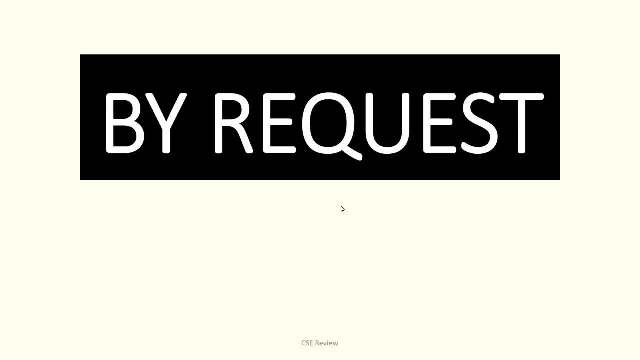 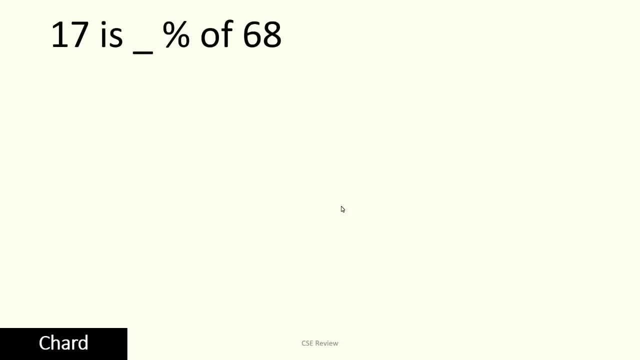 account. So if you would send it over to the official Teamlike Facebook page doon sa wwwfacebookcom slash teamlike instead. Okay, Alright, Let's start it. Let's get it started. Alright, Sorry about again, my voice Medyo ubos na kasi. 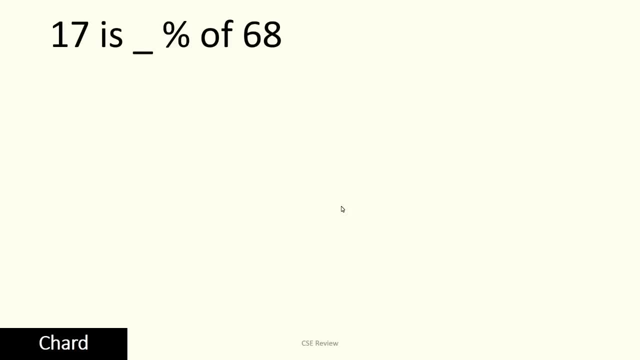 siya from teaching ng tuloy-tuloy and making all of these videos, But I do hope na intindihan nyo pa rin ako magsalita. Okay, So 17 is black percent of 68.. Actually I already made. 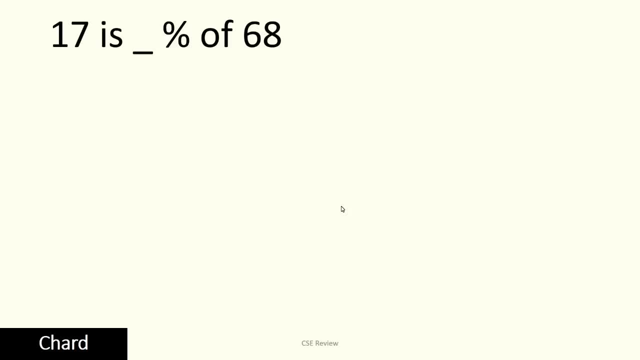 a series of videos on these topics So you can check out the percentages na series natin. But Charg sent this asking kung paano gamitin yung ratio rotation technique sa ganito specific na question, And I actually mentioned it a couple of times na rin in other videos. But I'm going to show you again kung paano. 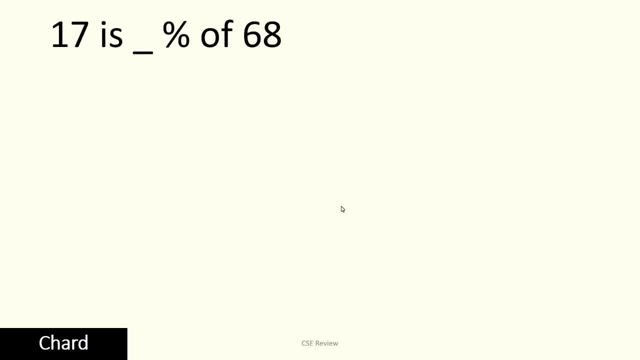 siya gawin. Hopefully you pick up the technique Now again. ang common na technique dito, or ang turo rin talaga in school, is: change is to equals and of to times. So ano yung ibig sabihin? nun, Ang formula niyan becomes seven, So you can see that the formula is. seven. So you can see that the formula is seven. So you can see that the formula is seven. So, if you start estimating for 18 and you find the 1, and then the total is 38 and then the remaining is 68.. Okay, That's your ruined strategies that you have to try to solve. So that's the basic method to solve for 18, and then the same, And then X, kasi ito yung nawawala, and then times 68.. Okay, So ito yung traditional method niyan. Okay, Tapos magsasort. 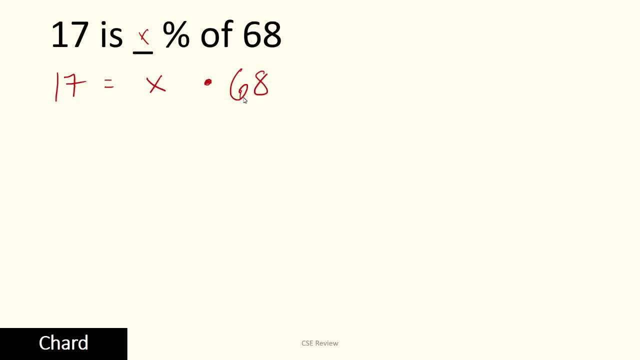 ka na na mag-solve for equalities Over 68 mo sila pareho. Okay. The problem with that is most of us allergic tayo sa division ng ganito, kasi obviously desima lang lalabas dahil nga percentage ang hinahanap. So another option would be to start estimating, or yung. 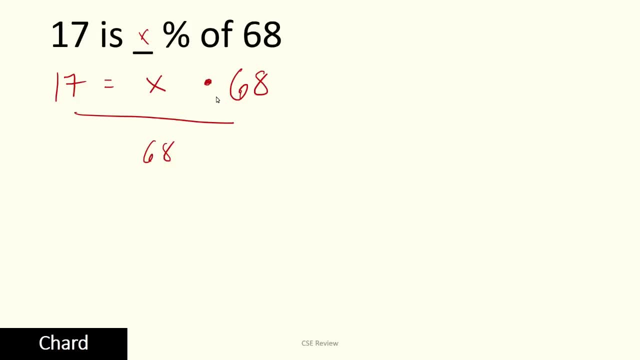 yung kiya tanong ni Charg ko paano gagamitin yung ratio rotation. So this is how you use. So this is how you use ratio rotation for this particular question, Yung 17,. meron tayong number side, meron tayong percentage side. 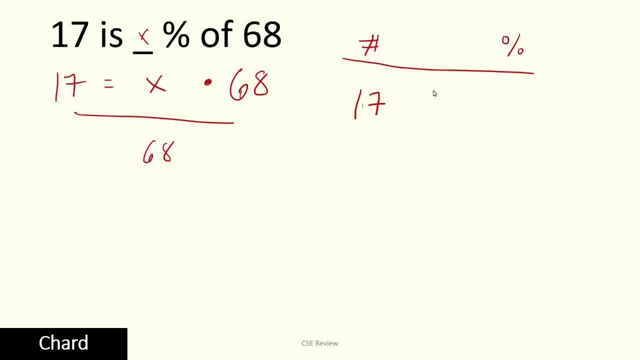 This is the same concept that I use for solving ng discounts And in that case, peso side and percentage side. Nandito, if you want to use ratio rotation, you have your number side, which is yung numbers natin, itong digits. 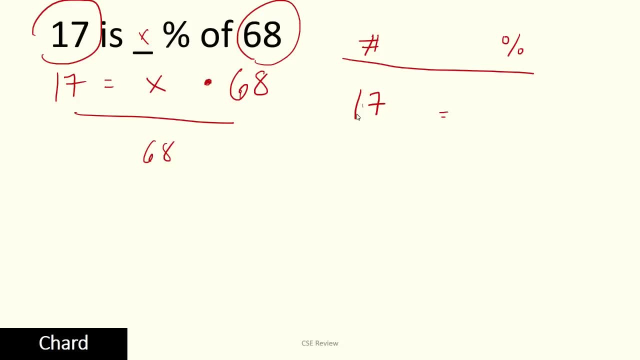 And then your percentage side, Now yung 17,. ano ba siya? 100% ba siya o yung percent na hinahanap? So obviously 17 is blank percent. So ang mangyayari katapat ng 17 is x, kasi kailangan magkatapat yung dalawang mga related na factors. 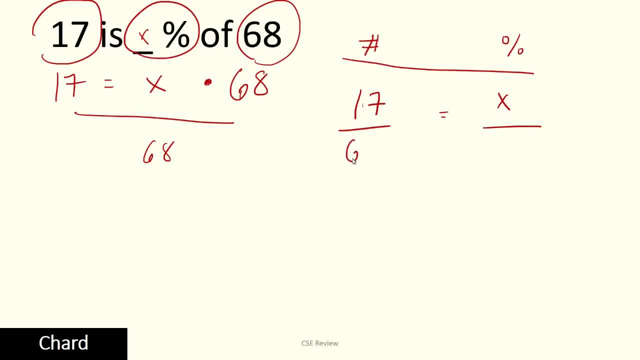 So 17,. katapat niya si x Yung 68,, which is also a digit, katapat niya naman yung 100.. Now bakit ito? automatic na 100%. Kasi yan yung original number. 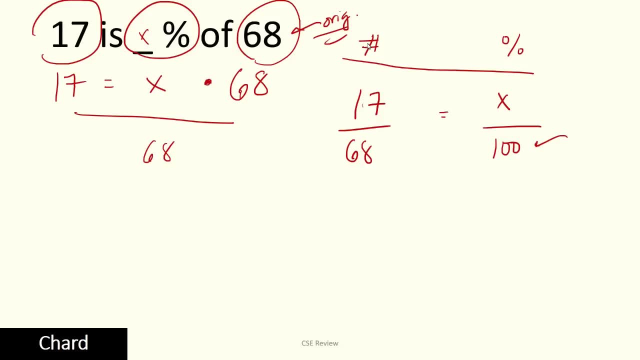 Yung original number. okay, Siya ang laging 100%. So that is what happens. Ito yung magiging ratio natin. Okay, So again you can start solving na using this and iikot natin siya. 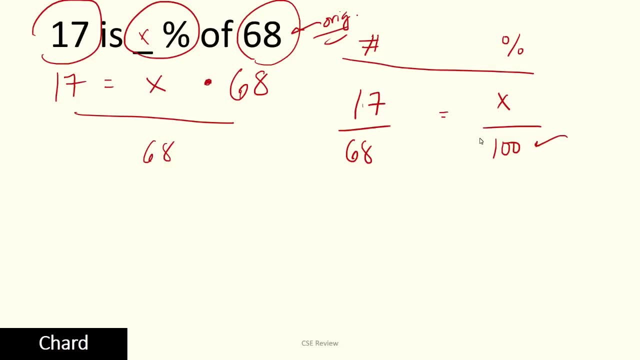 Now, in this case in particular, it's a little bit tricky, kasi yung 17,. okay, Hindi naman siya masyadong madaling i-factor, kasi prime number na yung 17,. no, Kaya you can actually start na by dividing it na lang right away. 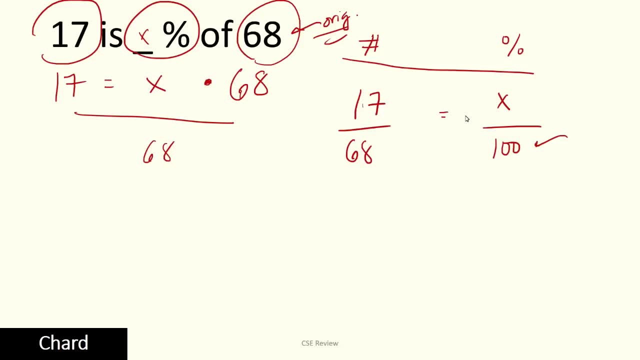 Yung productive to use ratio rotation pa in this one. Kasi nga ano na siya. eh, Mahirap na siya. i-factor. Okay Now, if you use the same technique, it's going to be the same din na output naman. 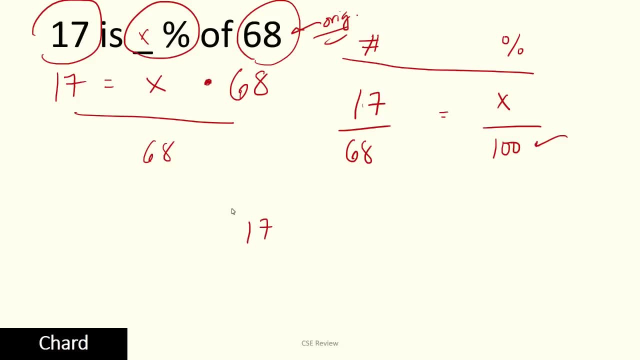 Baka maguluhan lang kayo lalo. So 17 na lang divided by 68, okay, What you could do would be to think of what you would do sa 17 para maging 68. siya, Instead of anong gagawin mo sa 68 para maging 17.. 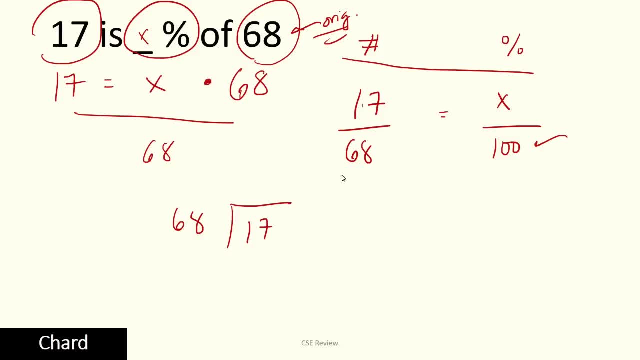 Kung meron kang mga options mas madali yan. Kasi, kung titinan mo yung 68,, if you divide it by 2,, okay, Ang lalabas is 34,. right Now, why did I divide it by 2?? Kasi, kung ano, yung divided by 2, yan yung times 50%. 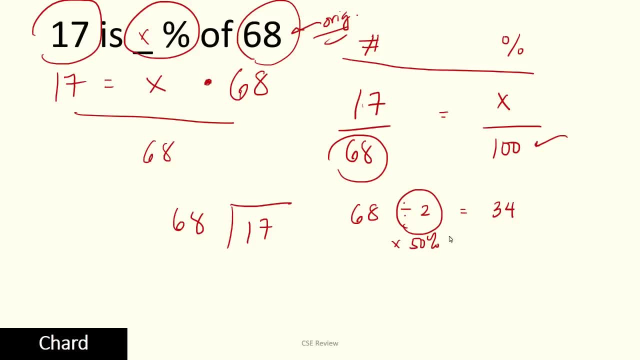 Kalahati. Okay, And yung 32 is 50% of the number, Ngayon yung 17,. if you look at it, comparing it dun sa 34, mo maliit pa masyado yung 17 dun sa 34.. 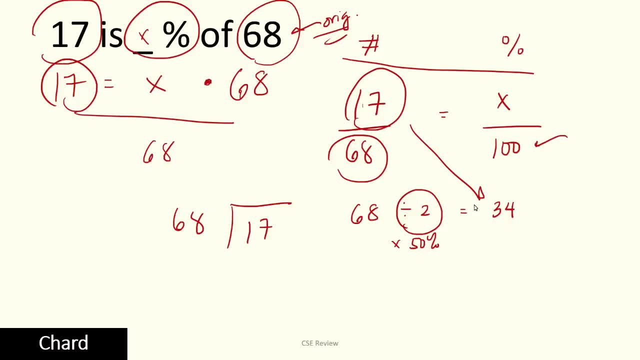 Okay, But you will start to notice yung relationship ng numbers right Mababa siya If babawasan ko pa ito ng gradually. okay, Kung gagawin ko itong kalahati ng kalahati or 25%, okay, 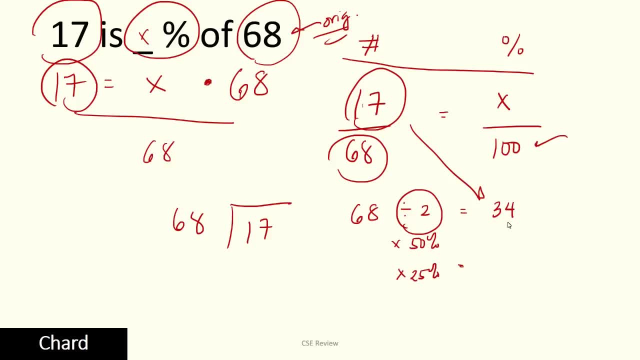 Ang 25% will be kalahati ng 50% And, if you notice, ang 17 kasi times 2 is 34.. So ibig sabihin nun, ang 25% is 17.. So again, ang sign here is to ang clue here. ang technique here is to try to find different ways, basta makuha mo yung tamang sagot. 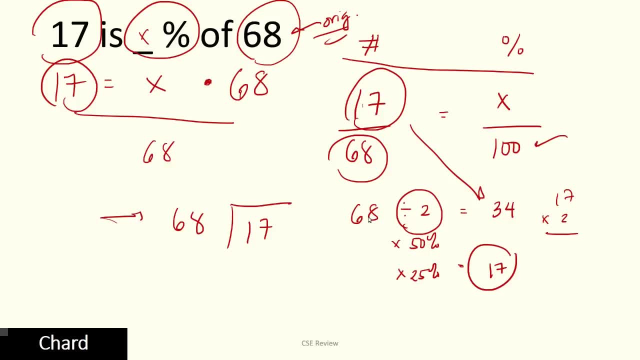 Kung ayaw mo talagang mag-divide, Okay. So if you notice, here again, ang 17 is 25%, So the answer here is 25%. Now, anong ibig sabihin? nun, Kung may options ka, you can just reduce and reduce yung numbers hanggang lumabas doon sa pinakamalaman. 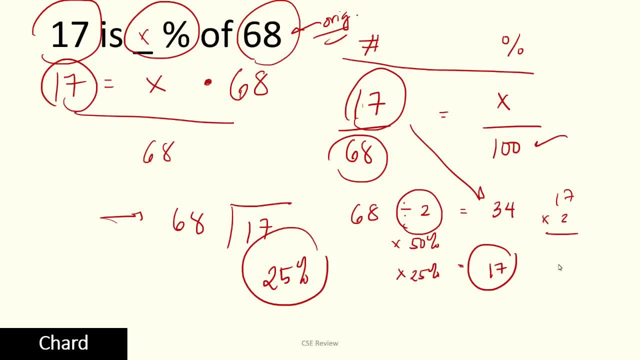 Ang pinakamalapit sa inahanap mo. Look at the options, Ano yung pinakamalapit Okay. So I just wanted to talk to you about that Para lang baka sakaling may mapulat pa kayo dito sa pagkakasolve ko. Okay. 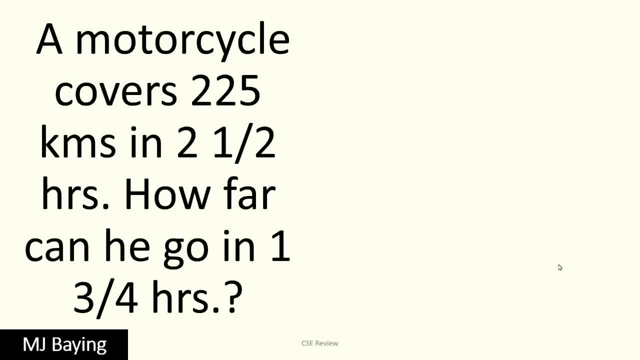 Now MJ Buying sent this Sabi niya: a motorcycle covers 225 kilometers in two and a half hours. How far can he go in one and three-fourth hours? Now, this kasi is a speed and distance na problem. 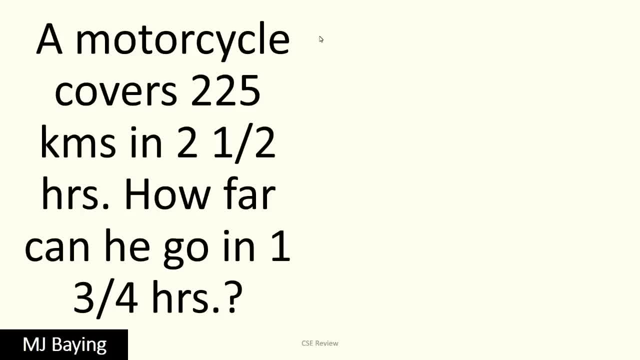 So you can start using yung speed, distance And time formula natin. So first step na gagawin mo is to find out the speed. Okay, Kung anong yung speed ng motorcycle. You can do it by dividing the distance over time. 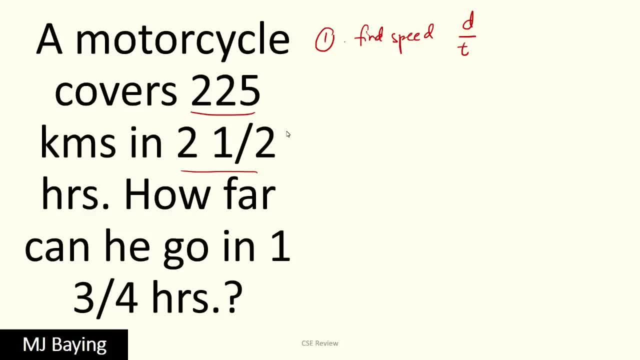 Which is yung 225 divided by two and a half hours. Next thing that you're going to do is you can find the distance by using the speed na nauna mong nakuha dyan. Now, the problem with that is it takes up time, So a lot of time. Ko-convert mo pa, i-divide mo pa yun. 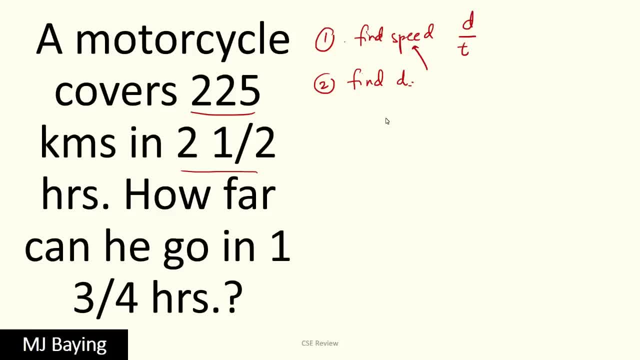 Di-mumultiply mo pa ulit dito, And so on and so forth. So there's something that I teach exclusively sa live review events, And that is how to use ratio rotation for these questions, Para hindi ka na dumaan doon sa formula. 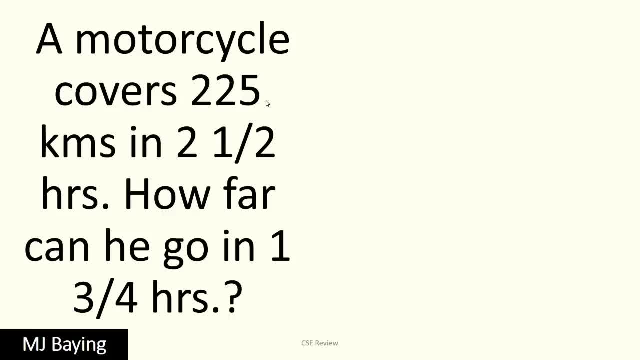 Ang gagawin mo lang. itatapat mo lang yung kilometer sa kapwa niya kilometer, hour sa kapwa niya hour. Bakit Kasi in this first sentence a motorcycle covers 225 kilometers in two and a half hours? Okay, 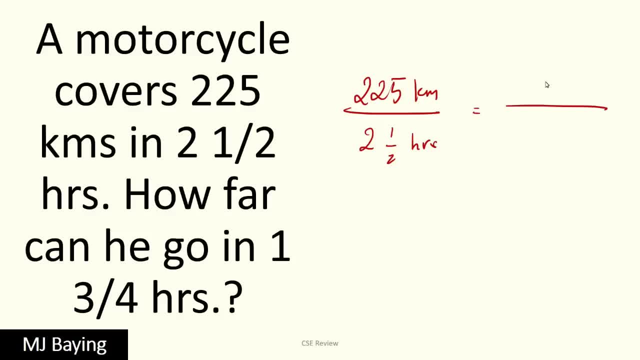 Tapos ang hinahanap mo kung ilang kilometer sa kapwa niya hour. Bakit Ang hinahanap mo kung ilang kilometers magiging x? Okay, Yung katapat na itatravel niya in one and three fourth hours Okay. 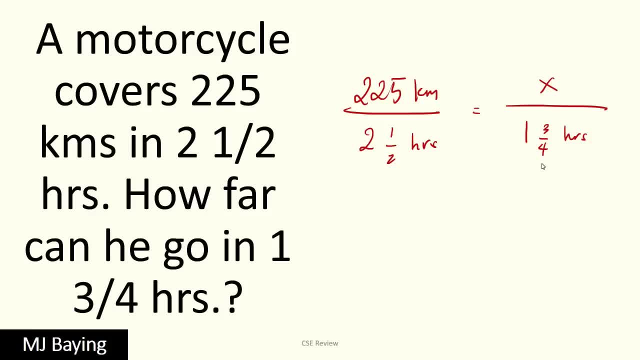 Now obviously mahirap yan. iikot kasi nga naka fraction form. Okay, And some people don't like using yung fraction form. What you could do would be to convert them into decimal, So 225, sorry, kilometers over 2.5 hours Okay. 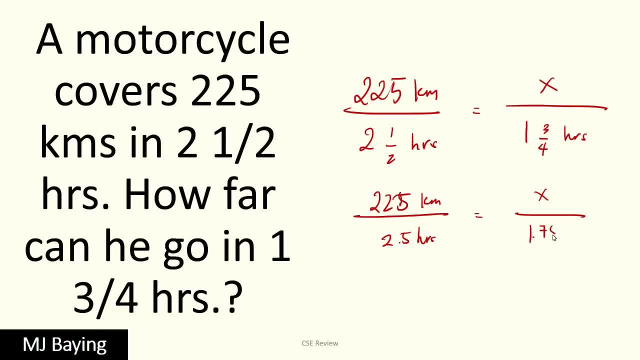 Equals x over 2.5 hours. Okay, Equals x over 1.75 hours. That is again if you're familiar with your decimal. Another option that you could do, if you really need that help, or allergic talaga kayo sa decimal- would be to change these into minutes. 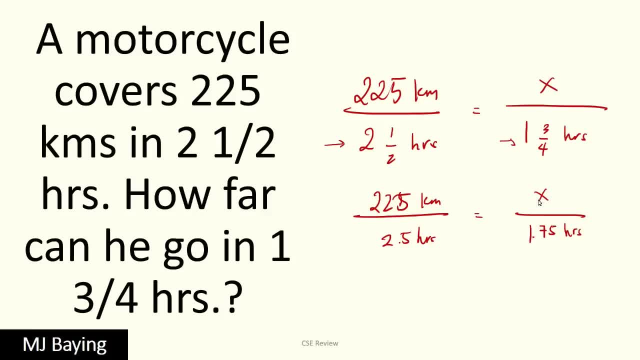 Kasi pag naging minutes yan hindi na yan magiging fraction or decimal Magiging. whole number na siya. So pwede mo rin gawing 225 over two and a half hours. So ang dalat ka lahating oras ay 150.. 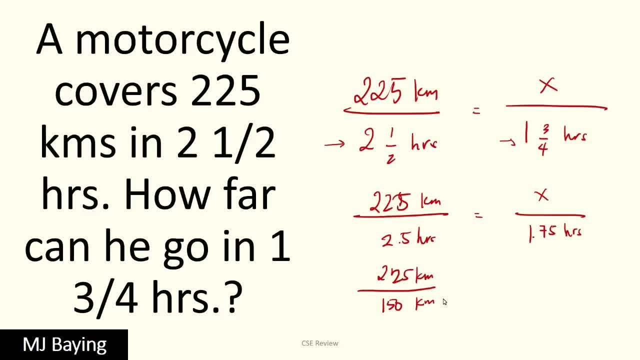 Yung mga hindi nakakaalam kung anong number yun Ang ginawa ko. that is just dahil sa isang oras may 60 minutes. Okay, So dalawang, 60 plus kalahati, which is 30.. Tapos dito x over, and then isang oras is 60 plus three fourth ng 60, which is 45.. 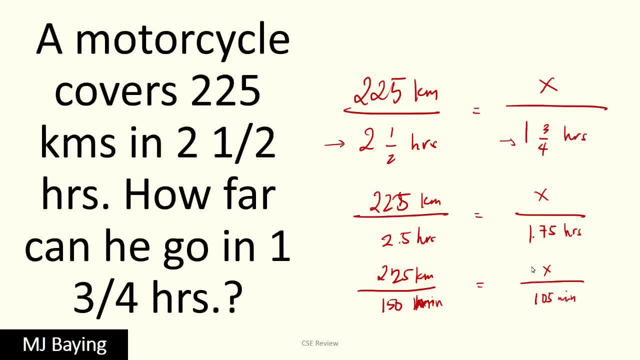 So that is 105 minutes. But the thing here, ang beauty nito, is all of those, kahit alin pa dyan, ang gamitin mo. Okay, You will come up with the same answer. Okay. So ano lang kailangan natin gawin. You just choose kung anong best na nag-work para sa inyo. 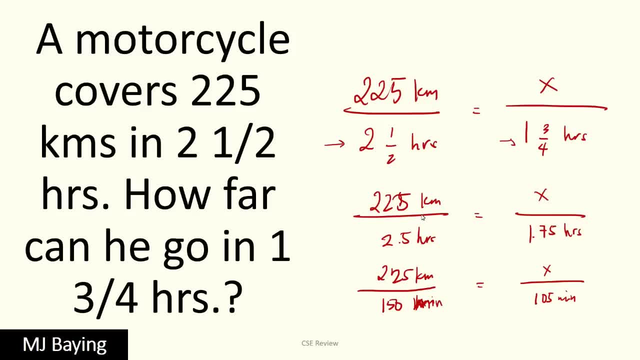 In my case. okay, I would rather use yung decimal Okay Here. It's not a big deal naman sa akin, So ang gagawin ko na lang would be 225 divided by 2.5, which is actually easy, kasi ano naman yan, pareho naman siyang divisible sa 25.. Okay, 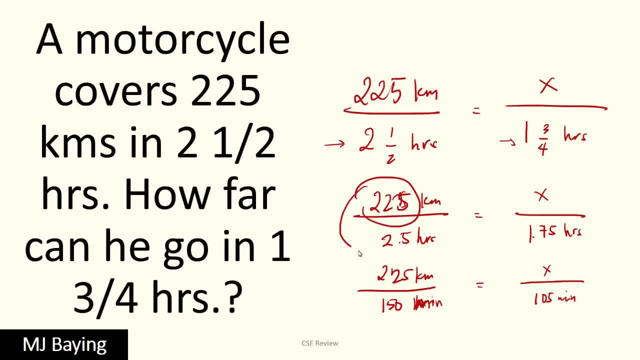 Okay. The answer here is actually going to be like this: Iikot lang natin ratio rotation 225 divided by 2.5, that will give you 90 times 1.75.. Okay, 90 times 1.75,. some people don't like solving yung decimals, nyan. Okay. 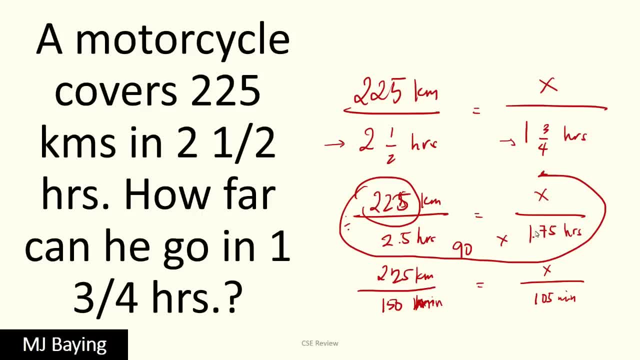 What you could do would be, if you want, okay, dahil meron ka ng 1, that is automatically 90. Tapos meron ka pang 0.75 ng 90. Okay, Which is basically 50% of it plus 25%. Okay, Or 0.5 and 0.25.. So ang kalahat is 45.. 0.25 is 22.5.. Ii-add mo lang siya lahat, Okay. 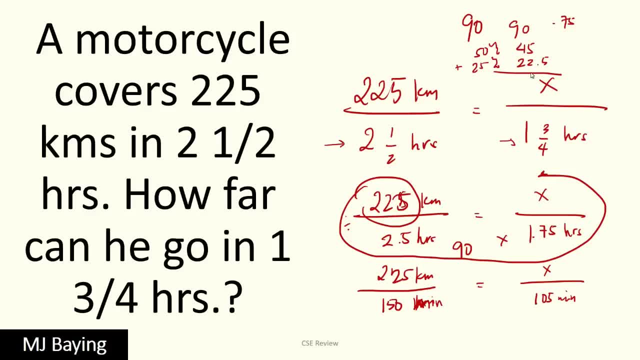 So I have 90 plus that, plus that, plus that. That is going to give you so 0.5, 7, and then this is going to give you 15.. Okay, So the answer is 157.5.. Okay. 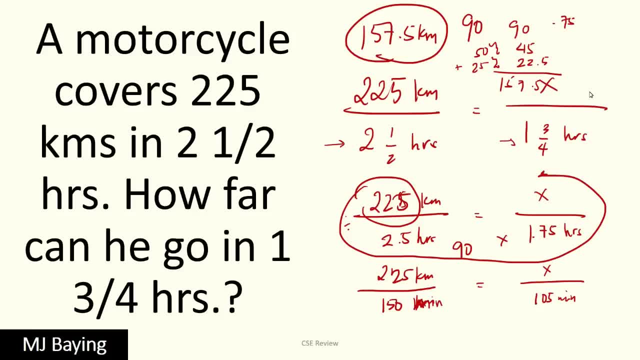 Now again, you can use that itong decimal. you can use this, kung Comfortable kayo with fractions: Kahit gamitin n'yo dito, you're still going to giv—It still going to give you the same answer, Okay. 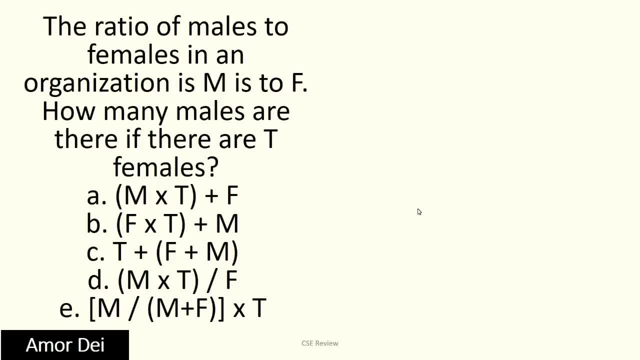 Next Eto The rates si region. naman si Anthony Amor, sor diya ma says: Y Okay, Why is this ratio problem? ratio problem, ito sabi ang male. ang ratio daw na male is to female is like that m is to f ang. 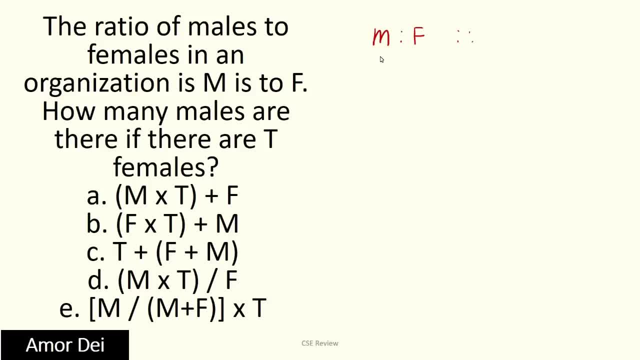 hinahanap is: how many males will there be? if there are t females, okay, so ibig sabihin nun, male, ang katapat niya dapat ay male din, pero ito yung nawawala, so yun yung nagiging x natin, okay, yun. 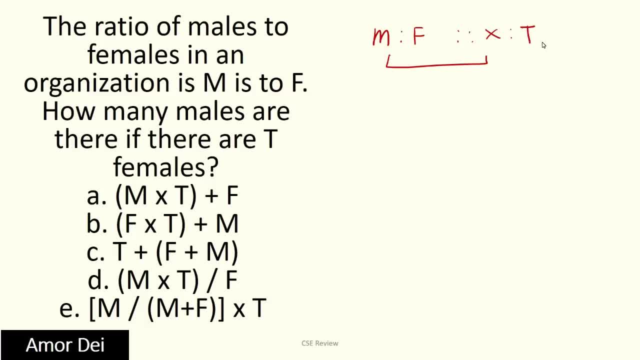 yung hinahanap natin. and then this becomes your t, which is yung the new number of females, kasi ang importante female katapat niya pa rin yung female, male sa male. so the fraction becomes m over f is equal to x over t. okay, tapos, anong gagawin natin? wag kayo matatakot kung letter lang sya. 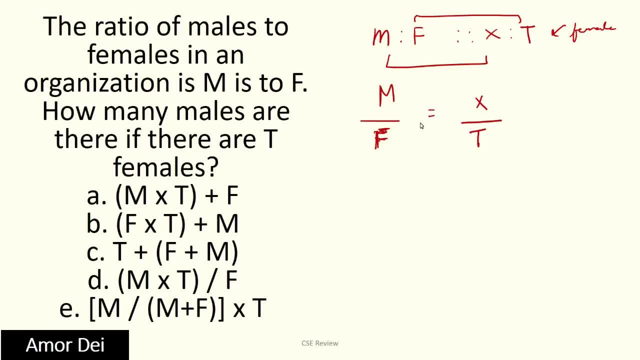 you're just going to do the same thing that you do with the numbers now in this case. okay, you cross, multiply it in traditional method: m times t is equal to f times x. and then, since ang hinahanap mo is the number of males, which is yung nilirepresent ng x, kailangan mong gawin: iwan yung isang, iwan yung x sa isang. 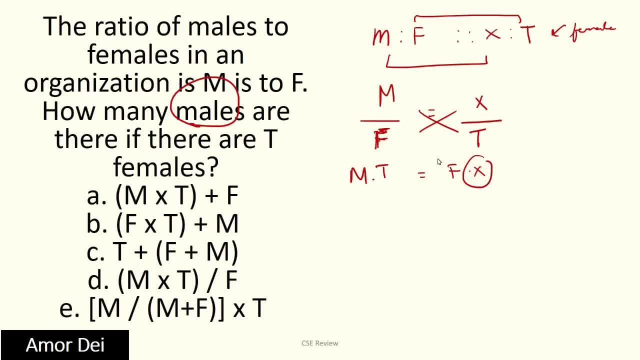 side okay. so parang mga totoong buhay na x. iwan mo sila sa isang side, layasan mo na sila. you divide both sides by f para makancel ito. so the answer is m times t over f. the answer is letter d, okay. 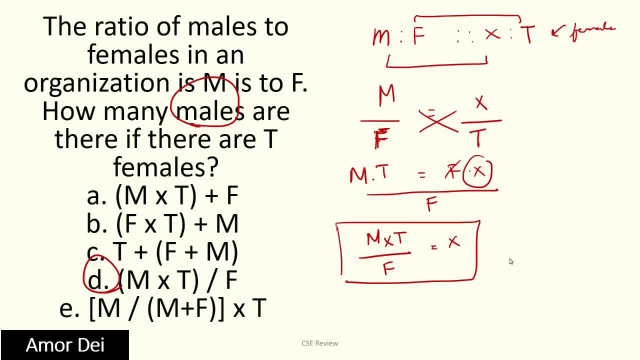 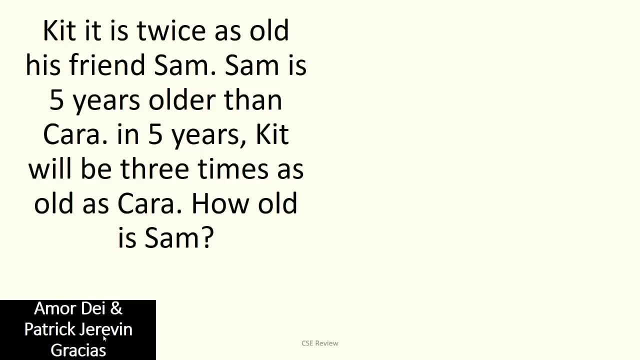 kasi yan ang equal sa x, which is the new number of males. again, tapatan lang yan, tapat, tapat lang ito. pidadala rin ni amore date saka ni patrick jerry pang graxias. actually this question was sent to me multiple times already. 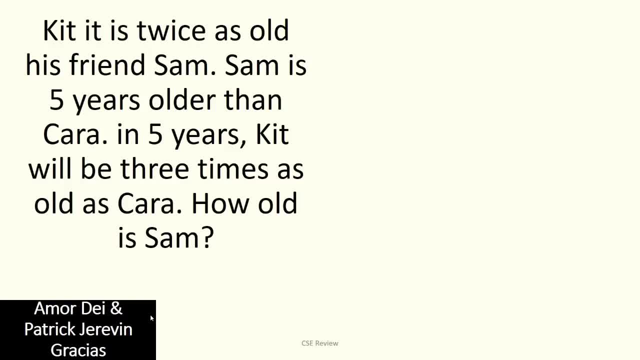 age problem, kaya naintindihan ko kung bakit maraming naguguluhan, and i'm going to try my best to solve this now. since walang options, hindi ko magagamit yung table technique na trial and error, so i'm going to have to use algebra. okay, again, when it comes to age problems, may video na rin ako nyan. 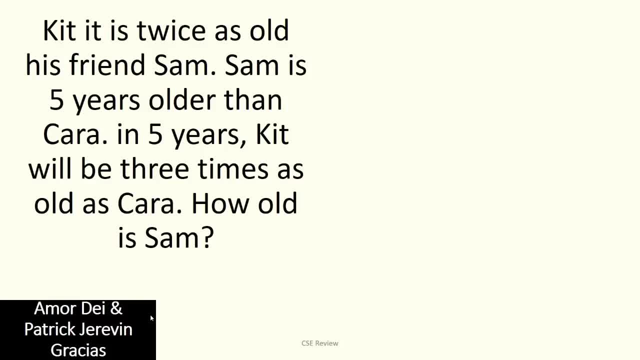 you can watch it. that is my method of solving this, if in case ayaw nyo talaga ng algebra at meron naman kasing options sa exam. so sabi kit is twice as old as his friend sam. sam is five years older than cara, so tatlo yung tao. 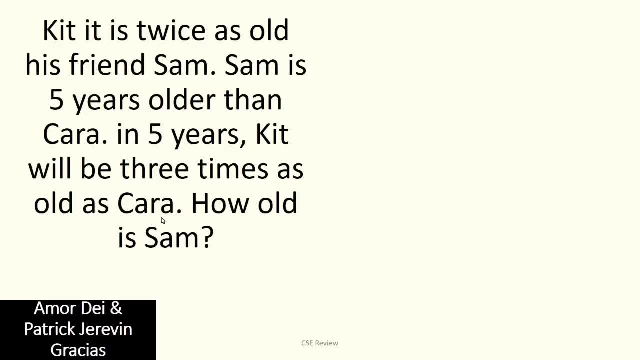 in five years kit will be three times as old as cara. how old is sam? now again yung techniques sa table. hindi mo magbabago, you have three people sa tatlo. ang rows mo one, two, three. okay, you have kit, sam and cara tatlo. sila ngayon yung time period natin ilan, so meron tayong is. 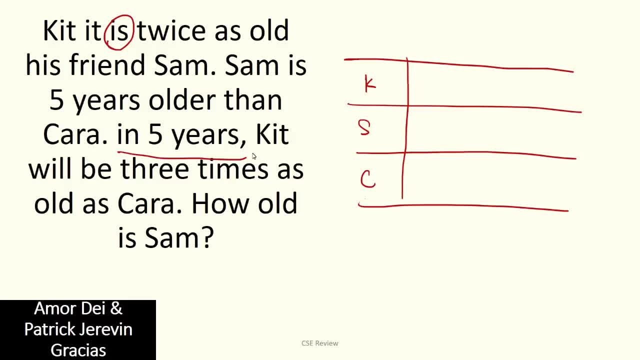 ibig sabihin may present tense: tayo. okay, meron tayong in five years. so meron tayong present, tas meron tayong future. wala naman ng iba. okay, so dalawa lang yung ating column. okay, you have. 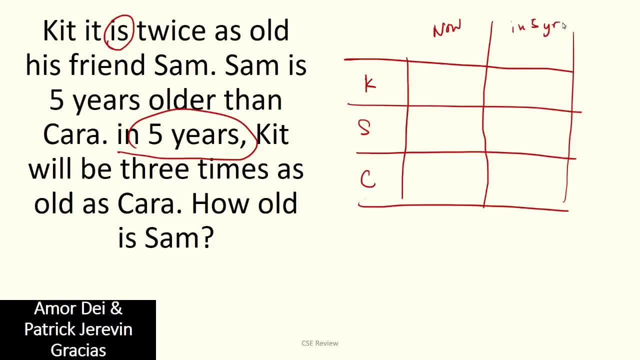 your now and in five years, again algebra. wala tayong choice, kasi wala siyang minigay na options. we're going to use our algebra ngayon. si sam ang hinahanap. so ibig sabihin nun, kung si sam ang hinahanap, siya yung. 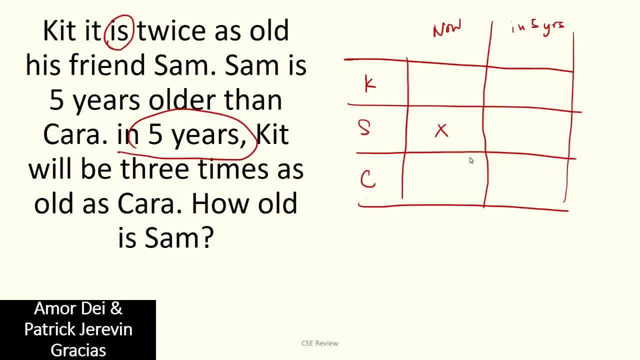 magiging x mo automatically. okay, ganun ang problema pagdating sa algebra, the next, or actually you can use something else, but magre-resolve ka ba, so i prefer na diretsyo ka na sa x. ngayon asabi kit is twice as old as his friend sam. ano ibig sabihin? nun? okay, si kit is older than. 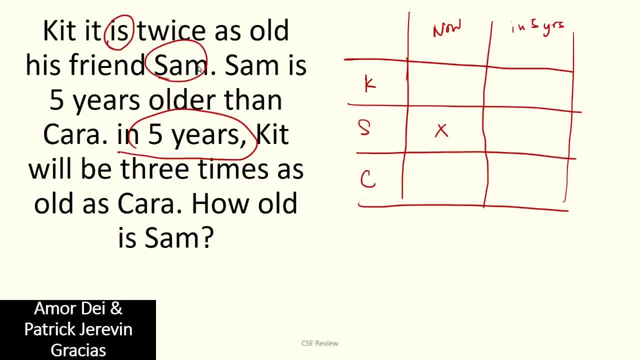 sam twice nung age ni sam. okay, para sinabi mo na ang edad ni kit ay doble nung edad ni sam. so kung si sam now, which is ang hinahanap natin ngayon is x, kit becomes 2x, next sabi: sam is five years older than cara. ano ibig. 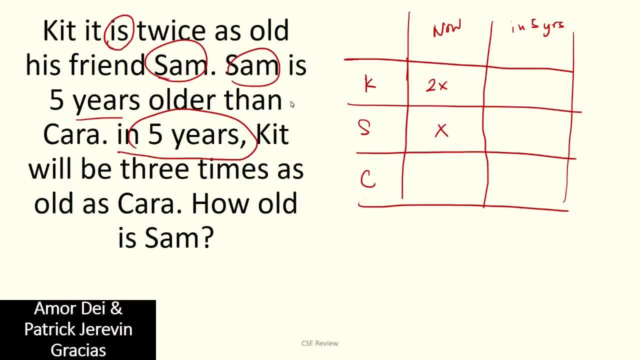 sabihin: nun mas matanda si sam ng five years kay cara. so kung naguguluhan kayo sa kung paano to i-convert into an equation, tagalugi natin and you use real ages, for example kung sam is five years older than. 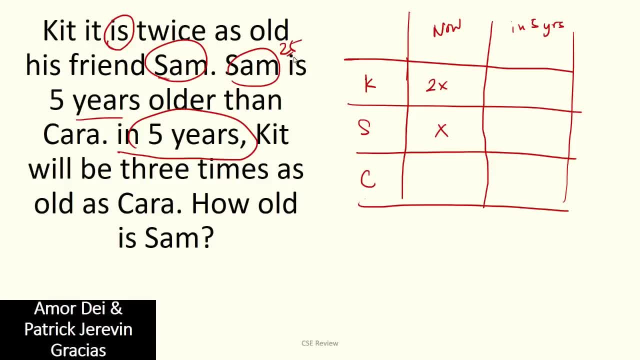 cara at si sam ay twenty five years old, siya y five years older. ibig sabihin si si cara will be twenty years old. anong ginawa natin sa twenty five para magiging twenty nag minus five tayo? so ano, ibig sabihin nun, to get Cara's age, that you're going to have to subtract five from. 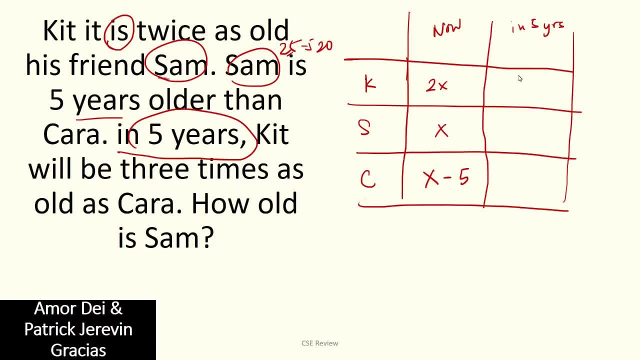 sam's age, so x dollars. So what does that mean? In 5 years we'll get the age of Kit. Now, every time we fill a column you'll add. So in this case, 5 years, that is 5. 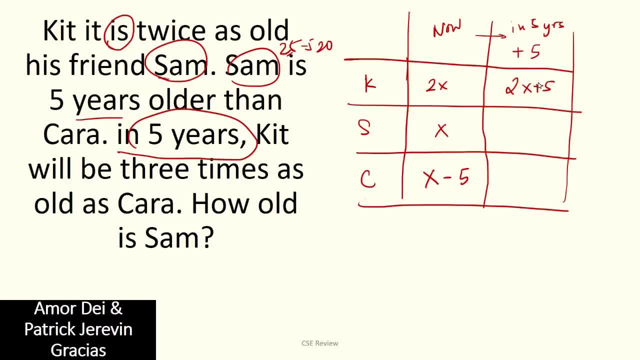 So 2x plus 5 is the age of Kit And it says we'll be 3 times as old as Kara. It means Kara x minus 5 plus 5, that is going to be x. Then our equation is that in 5 years, the age of Kit, which is 2x plus 5. 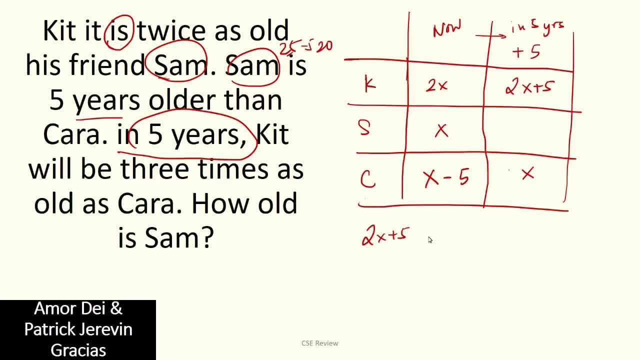 Is okay, or will be so equal. siya 3 times as old as Kara, So ano, yung age ni Kara: x. So that becomes our equation. So 2x plus 5 is equal to 3x. Okay, iiwan natin yung 5 dito sa side na to. 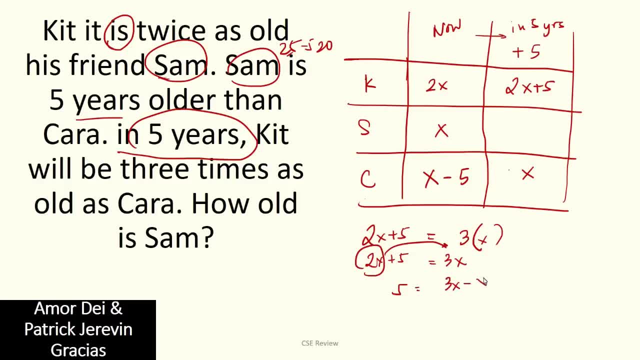 Ito ililipat natin sa kabila. 3x minus 2x is equal to 5, So 5 is equal to x. So the answer is x. Now, to check that I'm going to choose, Change my pen's color. 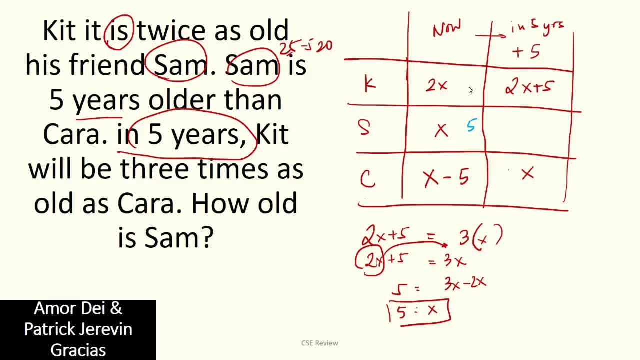 Kung gagawin natin 5, ang age ni Sam Kit becomes 10 years old, Si Kara naman is 0 years old, So ang age ni ibig sabihin na si Kara hindi pa siya pinapanganak Ngayong panahon na to. 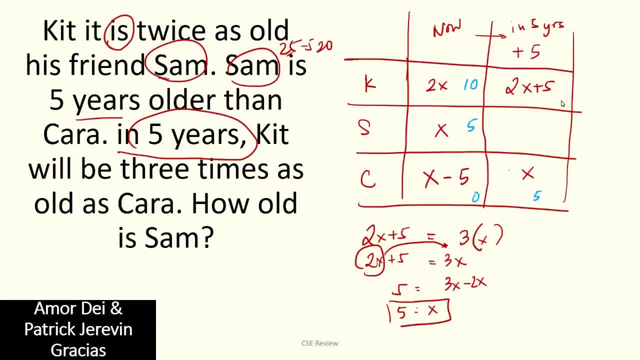 In 5 years, Kara will be 5 years old, Si Kit naman will be plus 5 niyan, which is 15 years old. So if you notice, 5 times 3, naman pa rin is 15, So it still works. 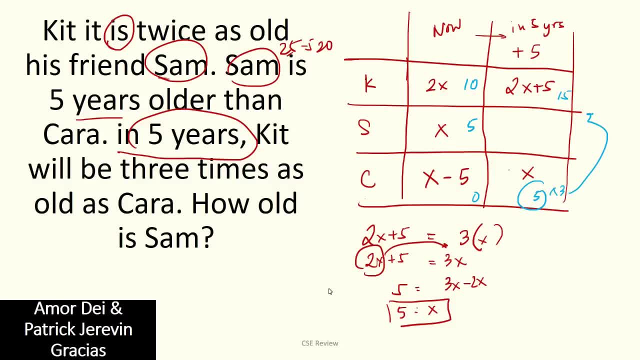 So the answer is 5 years Ngayon. there is a distinction here that I also want to point out. Nakalagay kasi dito, In 5 years Kit will be 3 times as old as Kara. Pag nakalagay yun na ganun. 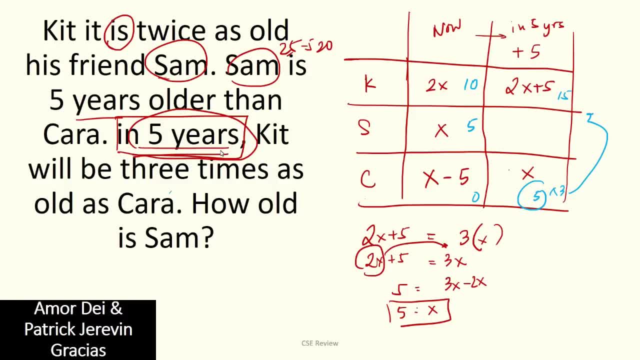 Ibig sabihin you have to assume Na kung ano yung time period na nalagay dito Is the same. Doon mo kukunin si Kit, Doon mo kukunin si Kara. I know probably dito maraming naguguluhan. 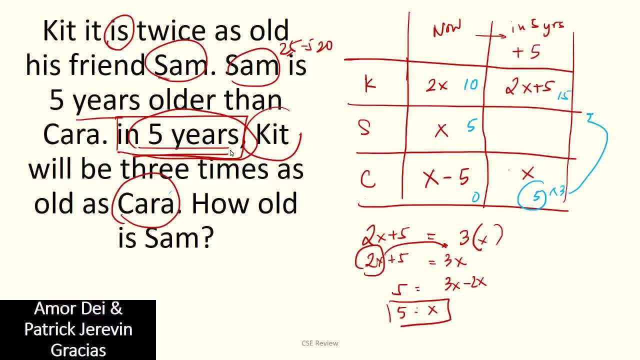 Okay, Now, if ang nakalagay is, In 5 years, Kit will be 3 times as old as Kara is today, O kaya as Kara's present age. Ang mangyayari nun would be: Ang imumultiply mo sa 3 is this: 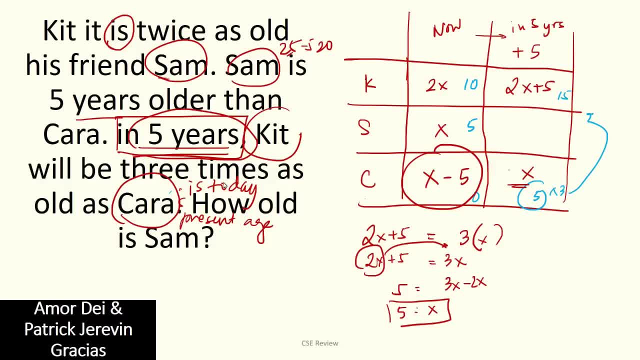 Not that, But since hindi siya nakaspecify At ang leading na statement nung sentence is in 5 years, You have to consider na ang Hinahanap mong age ay yung in 5 years. ni Kit at ni Kara. Okay, So the answer is 5 years old.